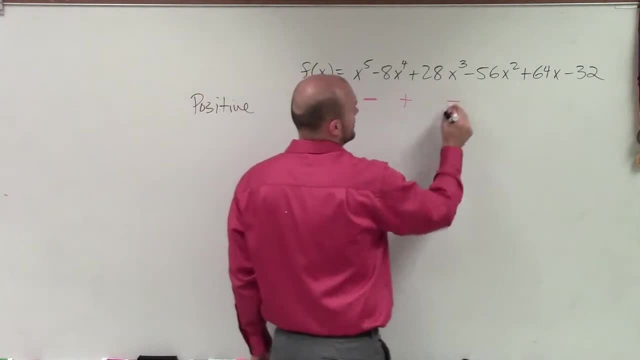 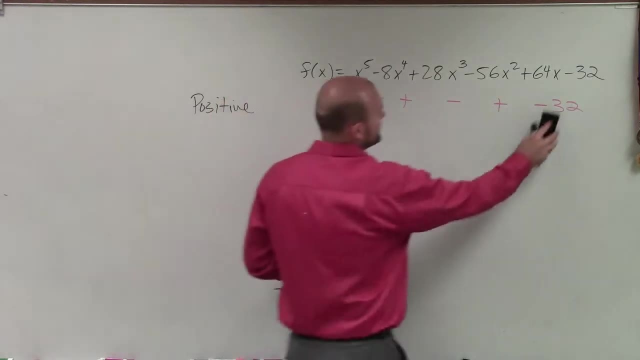 then I have a negative, then I have a positive 28, minus 56,, positive 64, and a negative 32.. Well, I don't know why I wrote the 32 in there. We just care about the sign, not. 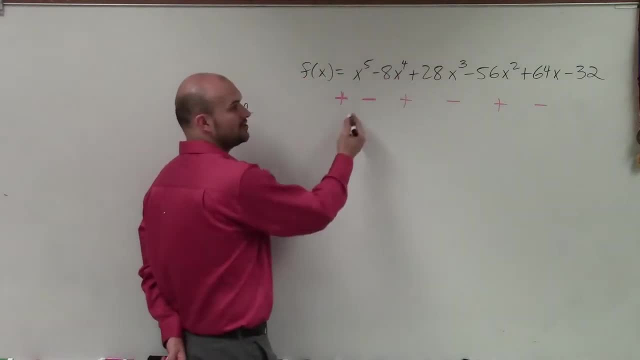 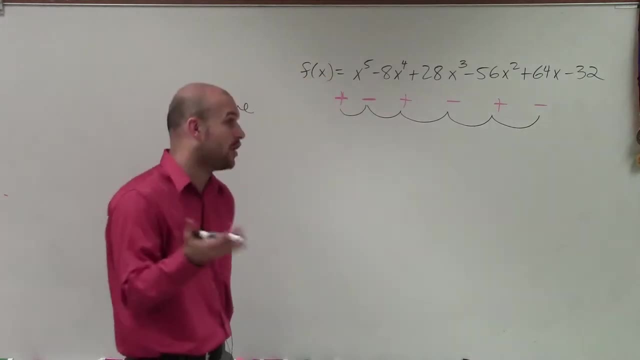 so much the numbers. So you can see my number of times that I alternate from positive to negative is 1, 2, 3, 4, 5.. So therefore, there's five alternating signs. We're going to use these as we say. So the number of positive real zeros is the number. 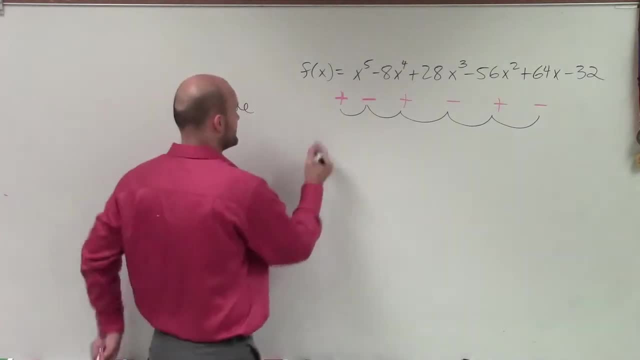 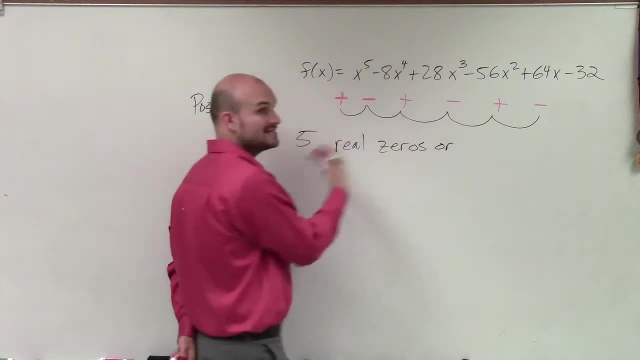 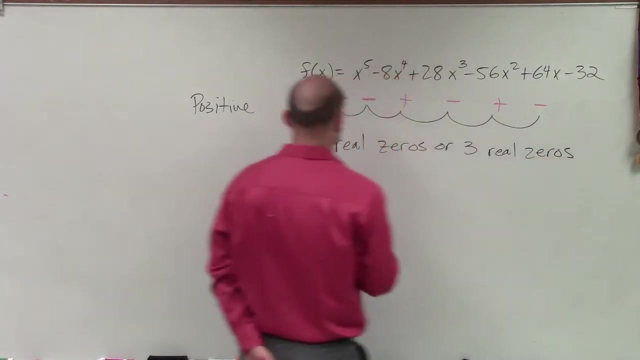 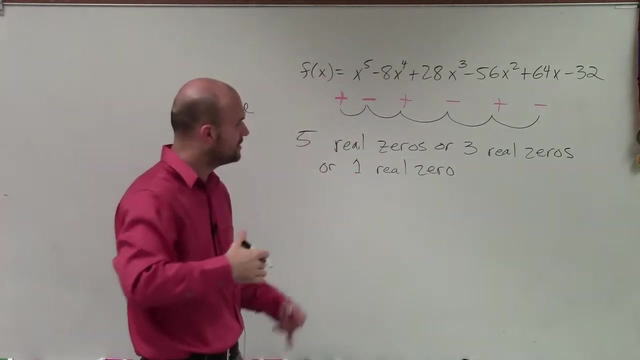 of times you alternate from a positive to negative, minus an even number. So you can say there's five real zeros or minus an even number would be three real zeros or one real zero. So you always have to include the total number of times you alternate and then keep. 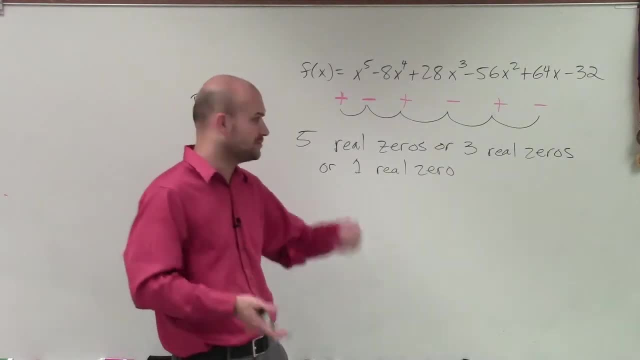 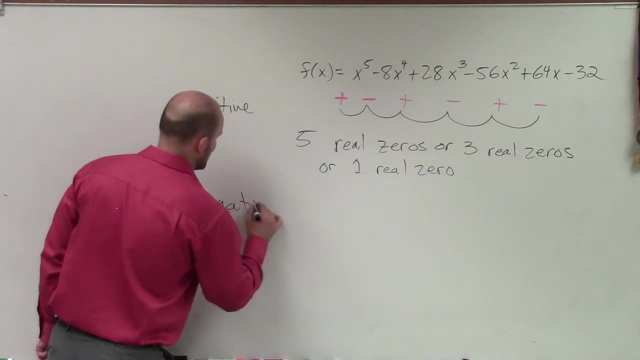 on subtracting an even number, and the easiest even number we remember is 2, and just keep on subtracting it so you can get all the possibility of positive real zeros. Now to determine the negative, I have to write out this whole polynomial again. So you have. 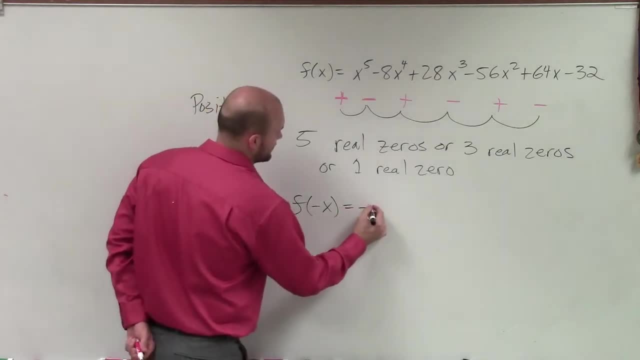 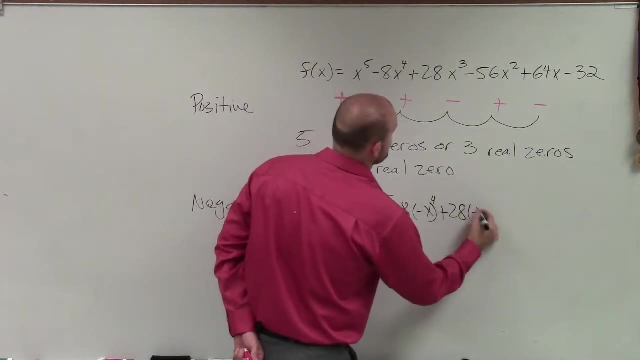 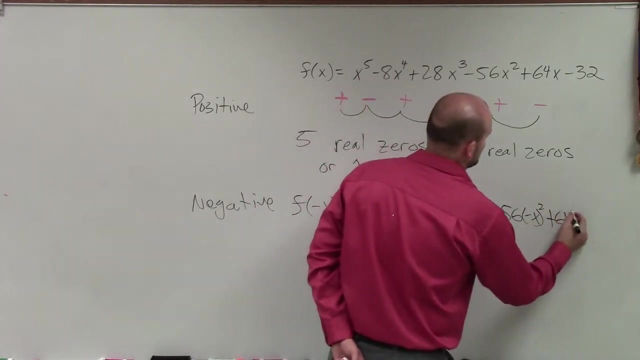 negative, which now you're going to apply in f of negative x. So therefore you have negative x to the fifth minus 8, negative x to the fourth plus 28 times negative x cubed, minus 56 times negative x squared, plus 64 times negative x minus 32.. So therefore negative. 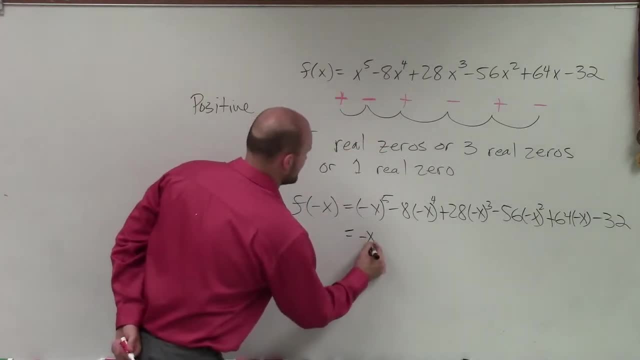 x, since it's raised to an odd power, that's going to become a negative. x to the fifth. Negative x to the even power will make it positive. times a negative will now be 8. x to the fourth. This is negative. x to the odd power will be negative and then times 28,. 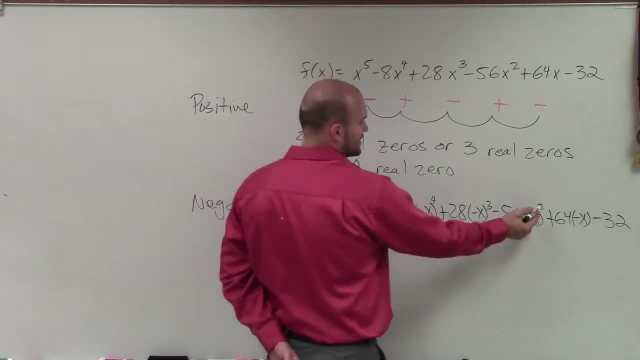 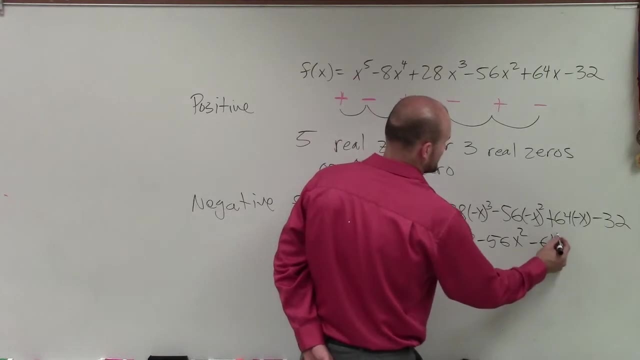 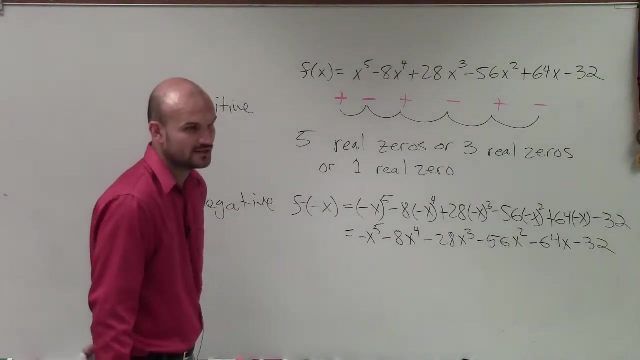 so that's a negative 28.. And x cubed, negative x squared, is positive times 56 is a negative. 56 x squared, This becomes a negative 64 x and then minus 32.. So, unless I made any other mistake, I'm not seeing any alternating signs, right? Because? 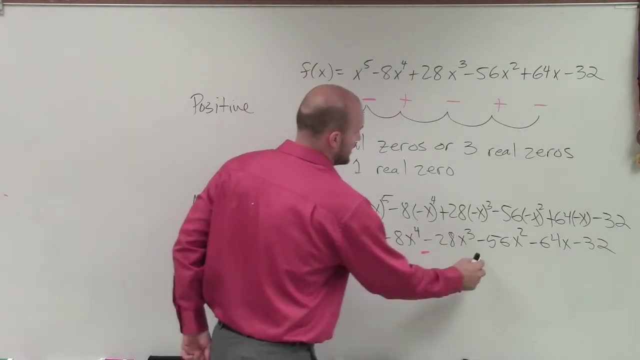 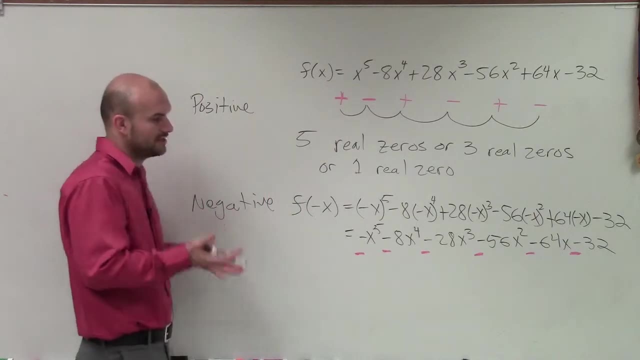 I bring down the signs, I have a negative, negative, negative, negative, negative, negative. Therefore, there's no alternating signs. So when I'm looking at my zeros and I look at the possible rational test, I know that none of my zeros are going to be negative. I have a possibility.